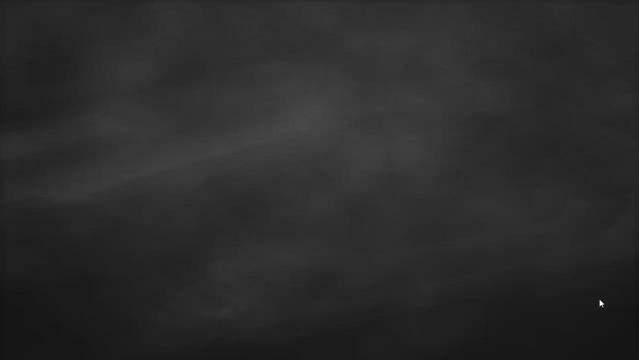 Let's get an example about supply and demand. So here we have the price 1,, 2,, 3,, 4, 5.. The quantity demanded at price 1 is 10.. If the price increases from 1 to 2, quantity demanded will be lower. so it 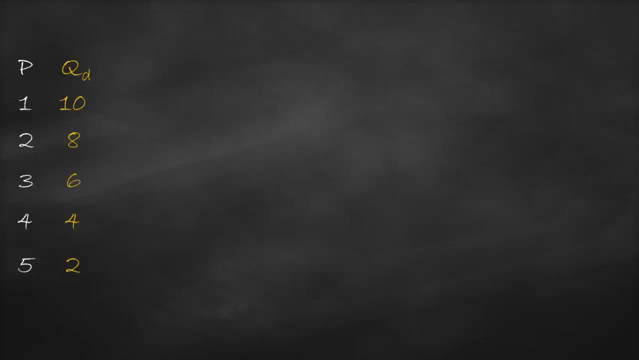 will be 8.. Then we have 6,, 4,, 2.. Quantity supplied at price 1 is 2.. If the price increases from 1 to 2, coin supplied will be higher. 4 and so on 6,, 8 and 10.. Let's draw both supply and demand, So our 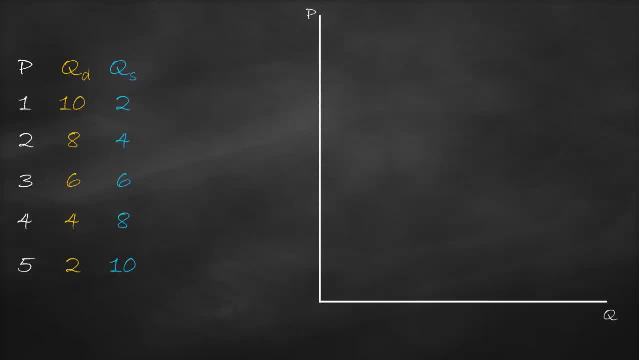 y-axis will be the price, x-axis will be the quantity and we'll put the tickers here: 2,, 4,, 6,, 8,, 10.. For the price, it will be 1,, 2,, 3,, 4,, 5.. For the quantity, demand at price of 1, we have 10 units. 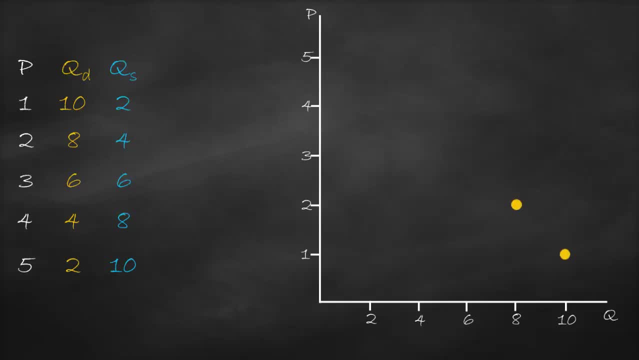 and then at price of 2. it's 8 units At price of 3, 6 units At price of 4, 4 units At price of 5, 2 units. Let's connect all the dots together, It will give us. 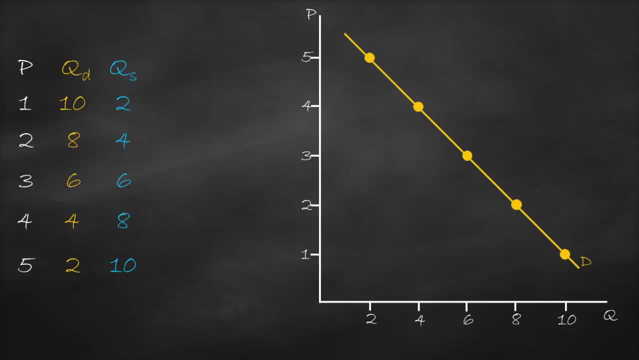 our downward slope demand curve. Why it's a downward slope? Because we have a negative relationship between price and the quantity demanded. If price goes up, quantity demanded will be lower, and vice versa. Let's draw the supply curve At price of 1, coin supplied is 2.. 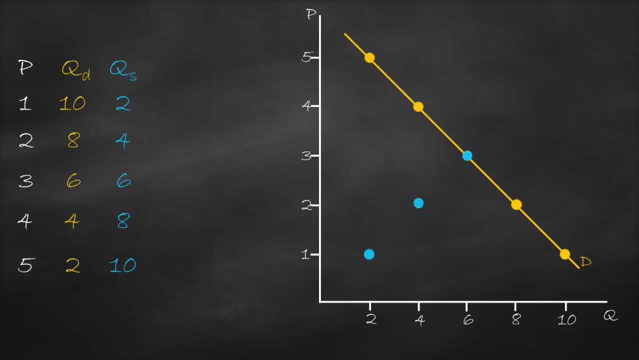 At price of 2, coin supplied is 4.. At price of 3, coin supplied is 6.. At price of 4, coin supplied is 8.. At price of 5, coin supplied is 10.. Let's connect all the dots together. This will give us our upward supply curve. 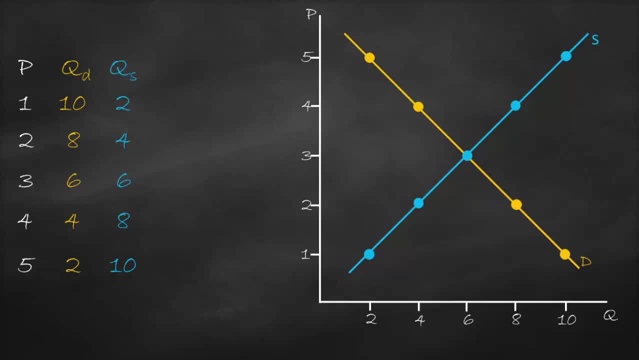 So let's look at the table first. Can you tell me where is our equilibrium point? So what do we mean by equilibrium? It means that quantity demanded is equal to quantity supplied. So if you look here at the table, you'll discover that at price of 3, our quantity demanded is equal to quantity supplied. 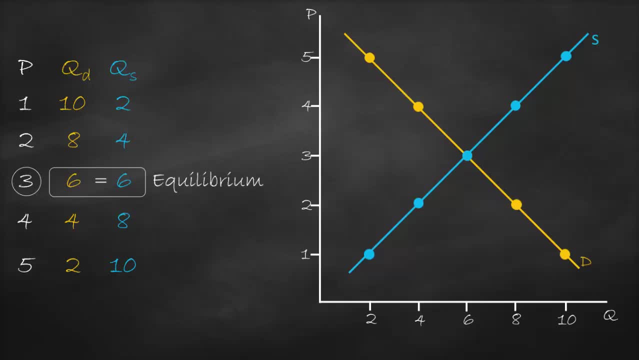 is equal to 6.. And that's why here we call it equilibrium. So our equilibrium price is 3, our equilibrium quantity is 6.. Why? Because quantity demanded is equal to quantity supplied. Can we get it from the graph? Yes, If you look here, where is the point of intersection between the supply curve and demand? 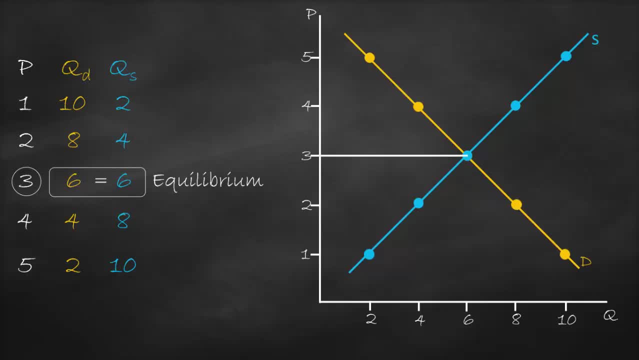 curve. It will be the point here where we have equilibrium price is equal to 3 and equilibrium quantity is equal to 6.. So this is our equilibrium quantity and equilibrium price. So we can get it either from the table or from the graph. So now let's look at the table. What will happen if we 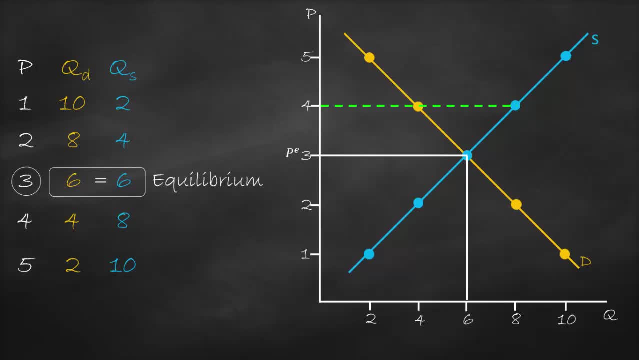 have a price level above our equilibrium price. Our equilibrium price is 3, but we'll have a price at 4.. So at price of 4, it will intersect with the demand curve and this will give us a quantity demanded of 4.. Then it will intersect with our supply curve and it will give us our quantity. 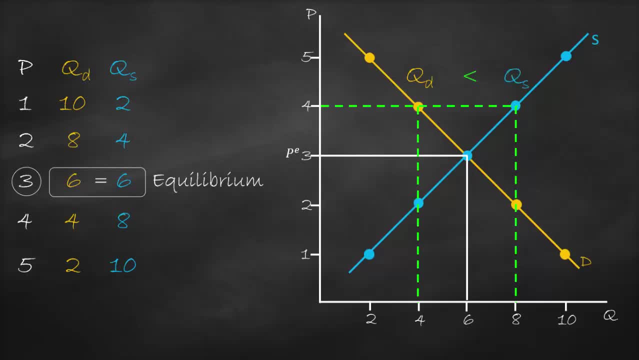 supplied of 8.. Therefore, we know that the quantity supplied of 8 is bigger than quantity demanded of 4.. Therefore, what is the difference between quantity supplied and quantity demanded? Quantity supplied 8 minus quantity demanded, 4.. So this means that we have excess supply, which means we have a surplus of 4 units. What will be? 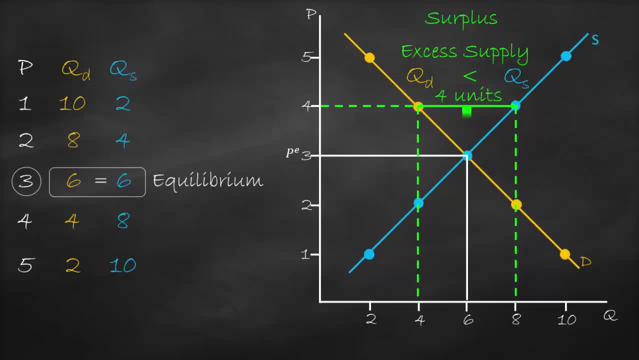 the impact of a surplus. Every time we have a surplus, this would result in lower prices until we reach equilibrium. Let's get an opposite example. What if we have a price level below equilibrium, For example, at 1.? Our equilibrium price is 3 and we have a price level at 1. It? 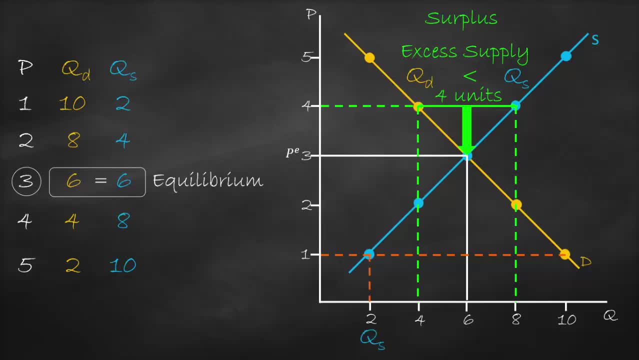 will intersect with our supply curve and we'll have a price level below equilibrium. So we'll have a demand starting at 0.. A demand starting at 1.. So at 1, X is equal to the demand curve. In other words, it will give us quantity supplied of 2.. It will intersect with the demand curve and 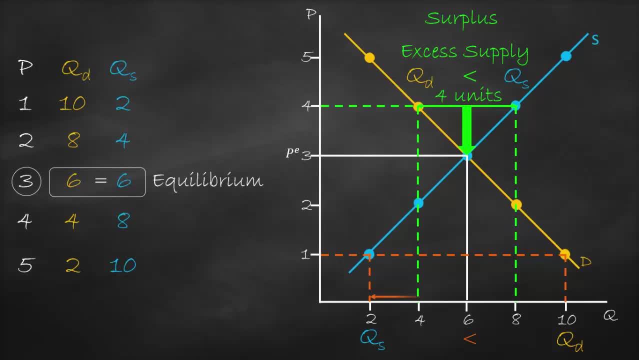 it will give us quantity demanded of 10.. I know that here quantity demanded is bigger than quantity supplied. of how many units? 8 minus 2 is 8 units. So this means that we have excess demand of eight units. Excess demands, it means that we have a shortage. So every time we have a 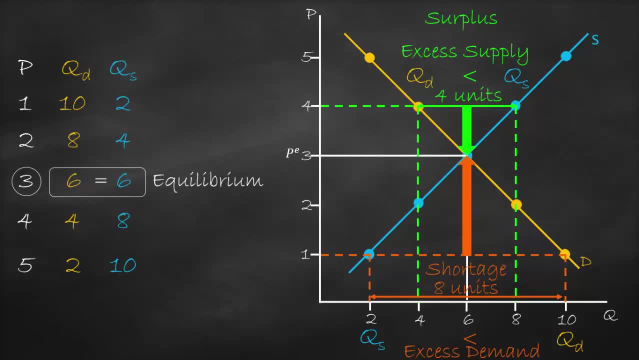 shortage. what will be the impact on price? Price will go up until we reach equilibrium, And this is what we mean by free market. It means that the market will increase and we will have an equilibrium. So we have a shortage demand. So we have a demand demand. We have a shortage demand. So this is the 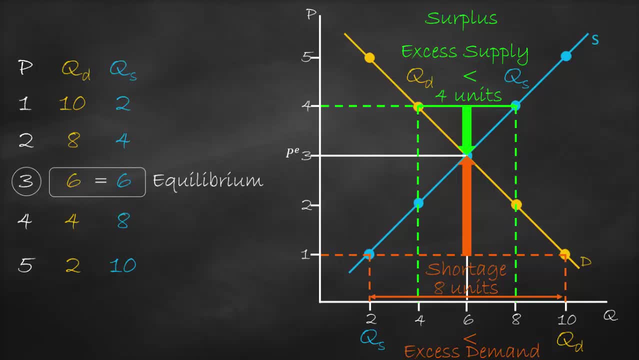 period of time. The line is that we have so many units, So we are going to have a shortage of units. So we market will correct itself by itself. if we are away from equilibrium, such as if we have a price level above equilibrium, it means that we have a surplus or excess supply. the impact: